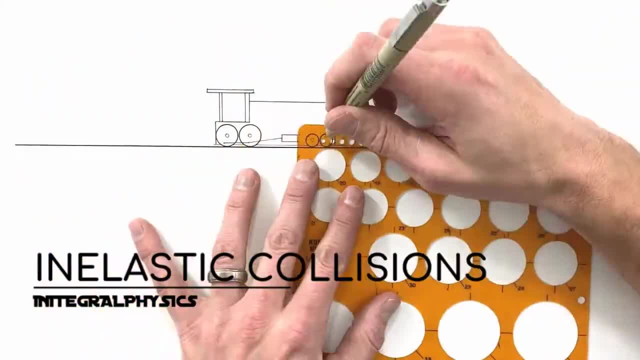 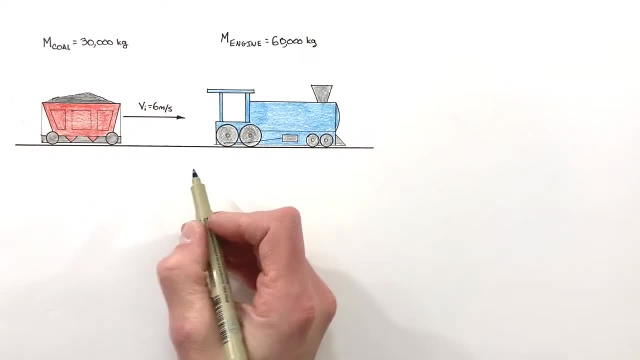 All right. what we're going to do today is take a look at the situation of a collision between a coal rail car and a steam engine, And so what we're going to set up here is really just an inelastic collision. We know that when a train car runs into an engine, these are going to couple. 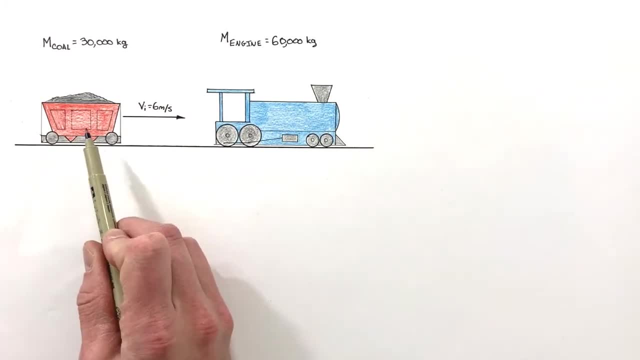 together, And so what we'll do is we'll have this coal car, traveling at six meters per second, initially slam into this engine. They're going to collide and stick together. Now the engine is initially at rest, And what I want to do in this problem is work out two different things: The 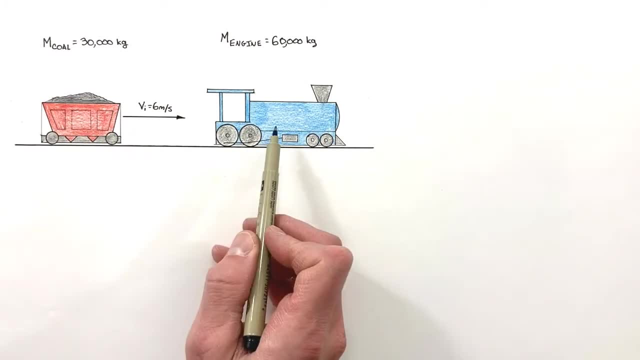 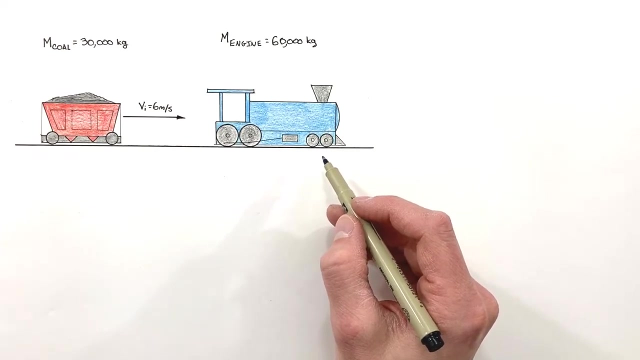 first thing I want to work out is the final velocity of the rail car and the engine once they've coupled together. Then I want to go through and look at the loss of kinetic energy in this collision. That is to say, I want to find out how much kinetic energy is lost to things like sound and 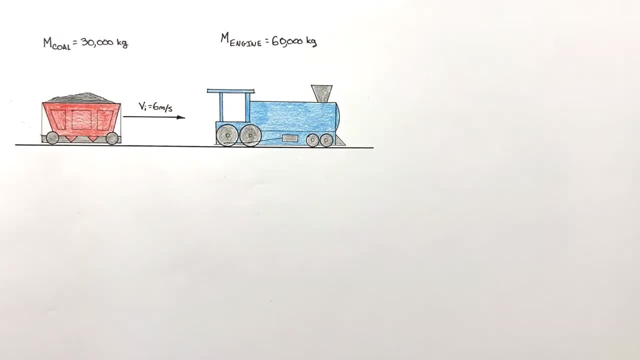 heat as this car slams into the engine. So first let's go through and work out the final velocity of these two once they've coupled together. Now we know this is an inelastic collision because the car and the engine are going to stick together. That makes them inelastic. Now, in any collision. 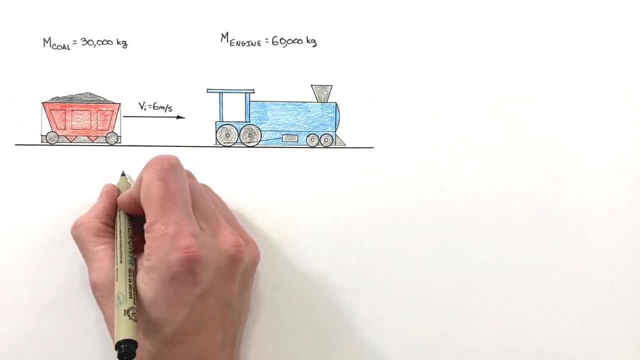 not just an inelastic collision, but any collision. we know that the initial momentum of the system is going to be equal to the final momentum of this system. Now, when I say a system, in this case I mean the coal car and the engine. So their initial momentums added together are: 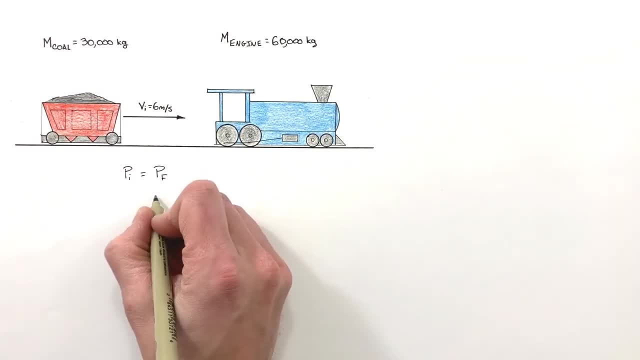 going to need to equal their final momentums added together. So let's first look at the initial momentum. We can look at each individual object and find its momentum and then add those together And that's all we're going to do here. So the initial momentum is going to be the momentum of 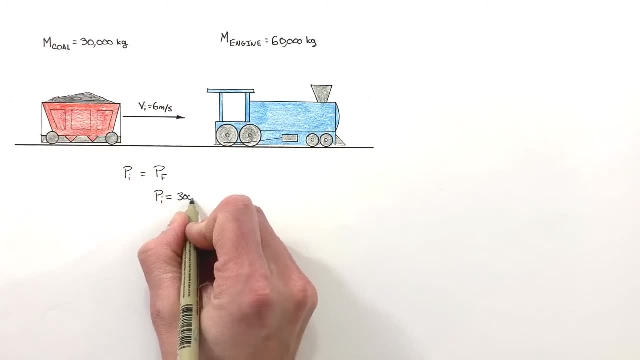 the coal car. Now we come up with something that's called the weight of the engine, And that's going to be 30,000 kilograms multiplied by the six meters per second which it is initially traveling, plus the mass of the engine, That's sixty thousand kilograms times zero. It's the initial 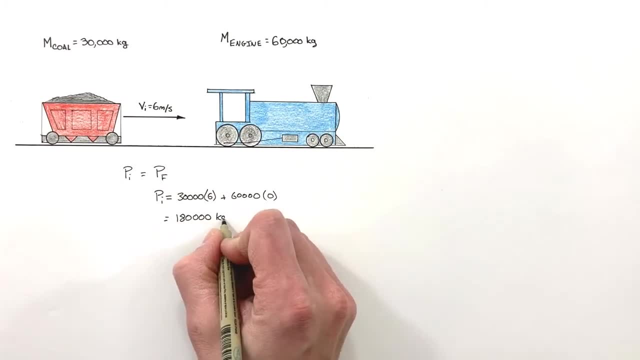 velocity And we come up with an initial momentum of one hundred eighty thousand kilogram meters per second. Now realize this is the initial momentum of the system and that total momentum will not change. So really all that's happening here is that we want to realize how big the engine can be and that total momentum cannot change. 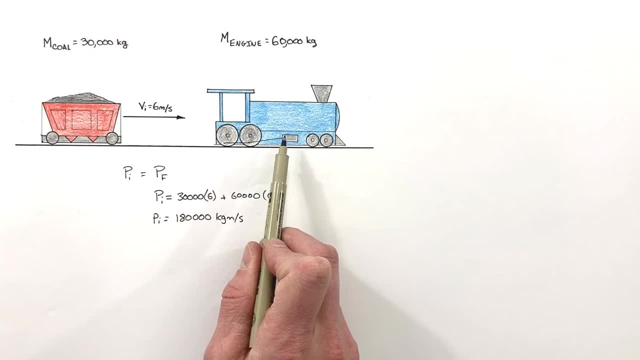 as this car slams into and then couples with this engine is. the momentum is simply being redistributed. So let's take a look at what's going on. in the end here, That's a P. We're going to pretend that's a P. In the end we have. our final momentum is equal to: 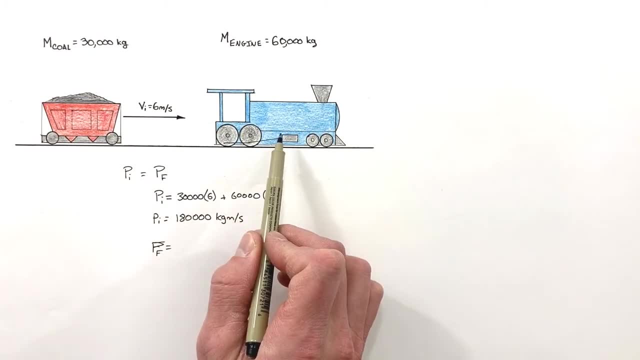 the momentum of each individual object. Now remember, if the car- here the coal car- has coupled to the engine, they're both going to be traveling at the same velocity, So our momentum in the end is simply going to be the sum of the two masses. 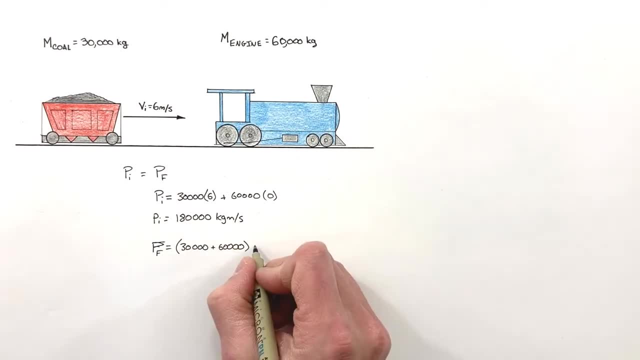 times their final velocity. We'll just call that V final. Realize, we simply add together the masses, because these two masses have coupled together and effectively become one 90,000 kilogram mass in the end here Now, in putting all this together, substituting in P I and P F, we get 180,000. 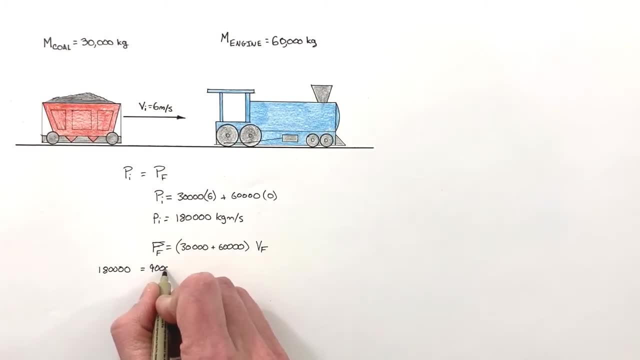 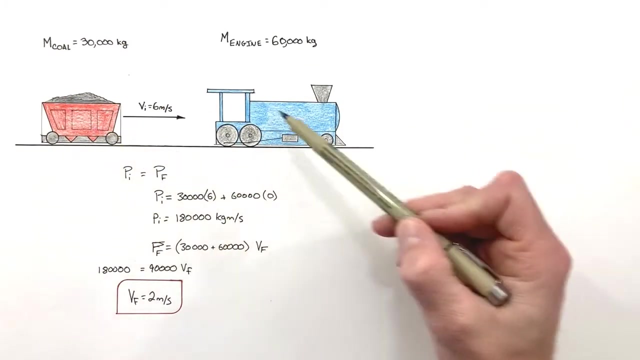 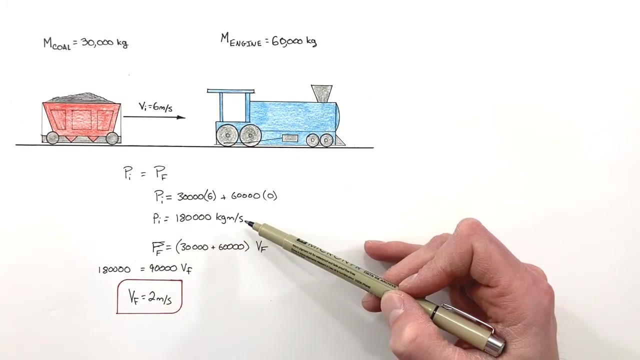 is equal to 90,000. Times V, F, And this leaves us with the final velocity of two meters per second. This means, after the collision, once the car and the engine have coupled together and are effectively sharing this, 180,000 kilogram meters per second worth of momentum. the coal 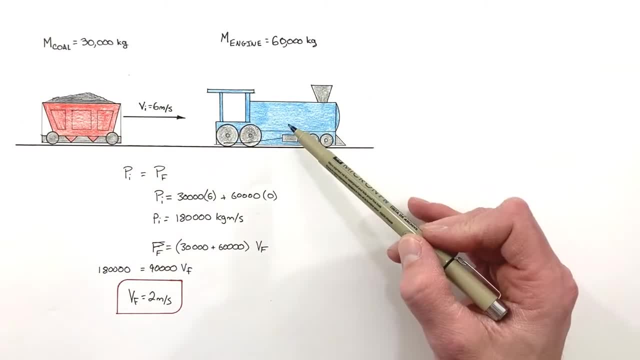 car will have slowed down some and the engine will have sped up and they'll both be traveling along at two meters per second. It's critical that we understand that in an inelastic collision the final velocity of both objects is the same. That is critical to solving the problem. 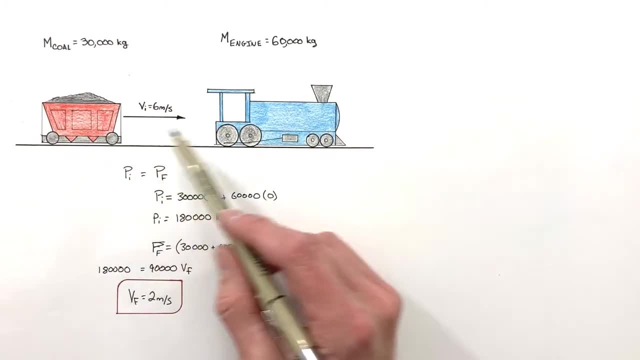 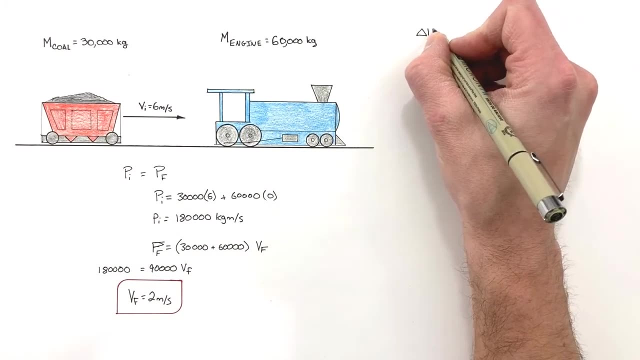 Now another big point to make when dealing with inelastic collisions like we're seeing here is what happens with kinetic energy. So what I want to go through and do is solve for the change in kinetic energy in this collision. Now we know change is given by final, So in 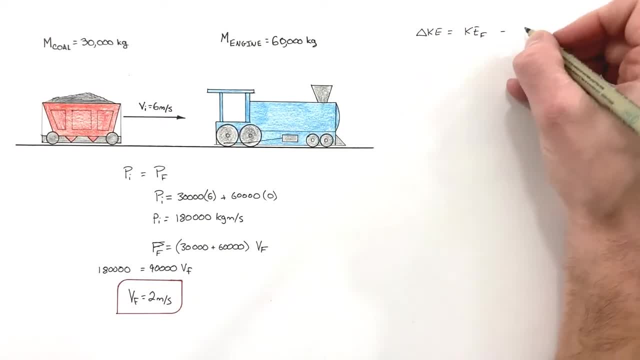 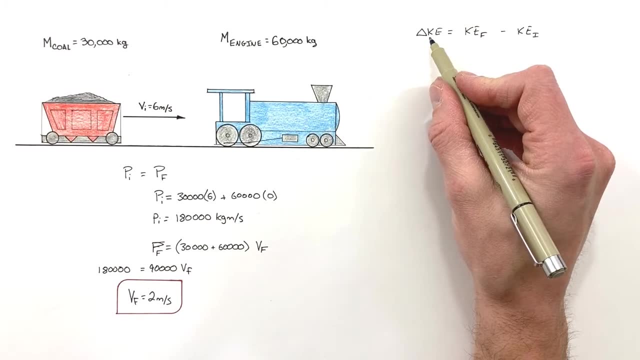 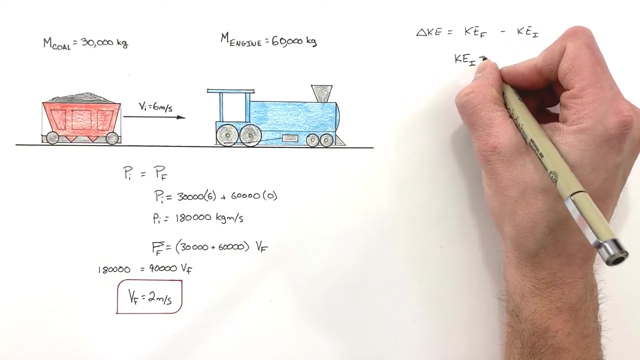 this case that'll be final kinetic energy Minus initial, In this case initial kinetic. So if we can find each of these values, we'll be able to find the overall change in kinetic energy of the system, Starting with our initial kinetic energy Initially. just this coal cart is moving and 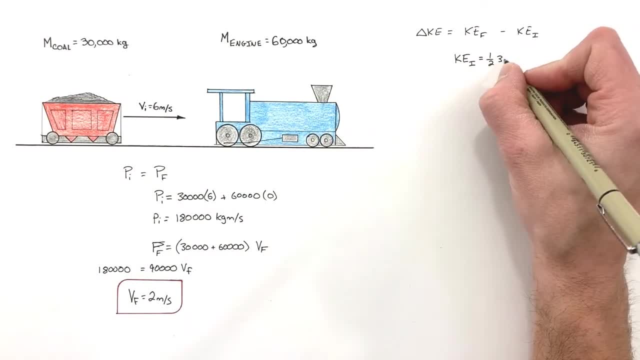 looking at its kinetic energy, we have one half times its mass, That's 30,000 times its initial velocity. That's six squared One half MV squared Plus the initial kinetic energy of this engine. Now the engine is initially at rest, so that's. 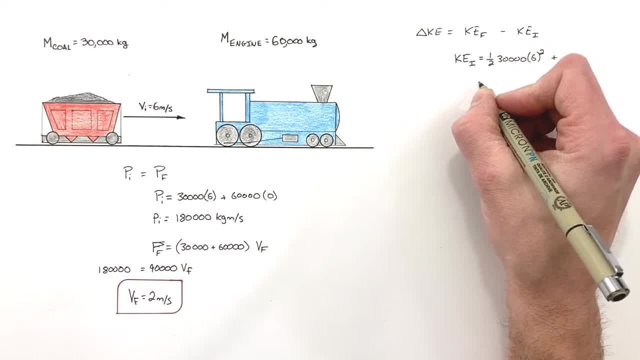 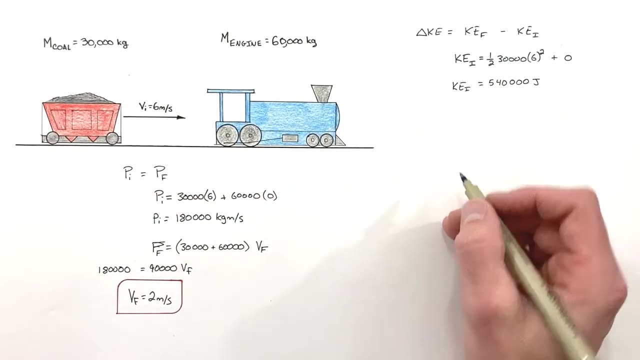 just going to be zero. Now this works out to be an initial kinetic energy of 540,000 joules. Now it's tempting to say, because momentum was conserved, we can also expect energy to be conserved. But watch what happens here. Let's work out the final kinetic. 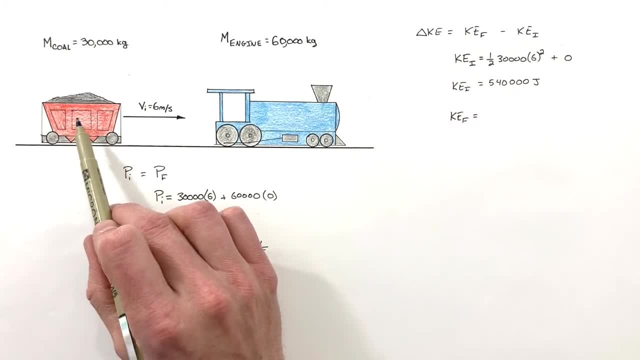 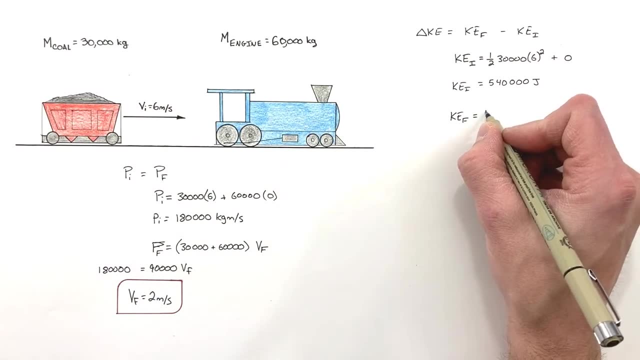 In the end of this problem we have the 30 kilogram, a 30,000 kilogram railroad car and the 60,000 kilogram engine both moving together. So really what we have is 90,000 kilograms moving along at two meters per second. So looking at kinetic, 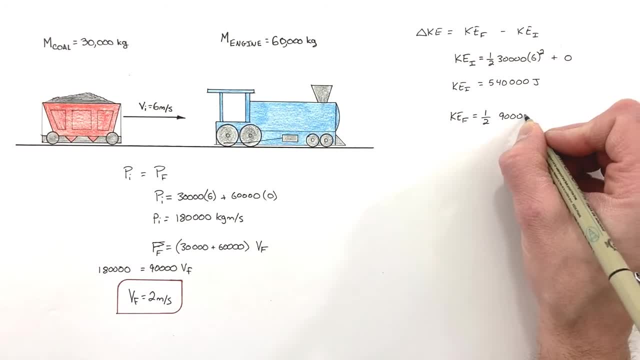 energy we're going to have one half times 90,000.. That's our total mass And all of that mass is moving at two meters per second squared. We already solved for this two using the conservation of momentum And this works out to be a final kinetic energy. 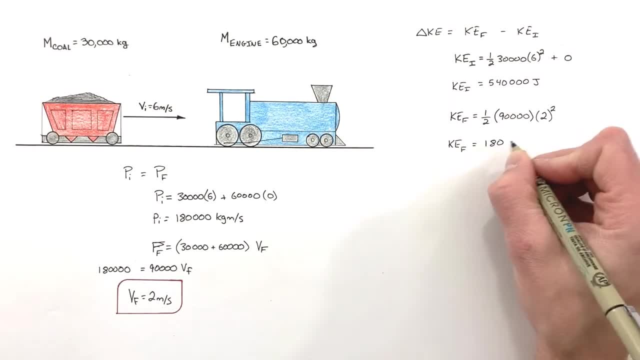 Minus initial kinetic energy, Minus initial kinetic energy, And that's the final kinetic energy Equal to 180,000 joules. Equal to 180,000 joules. You can see we started with 540,000 joules of kinetic energy and we finished with 180,000. 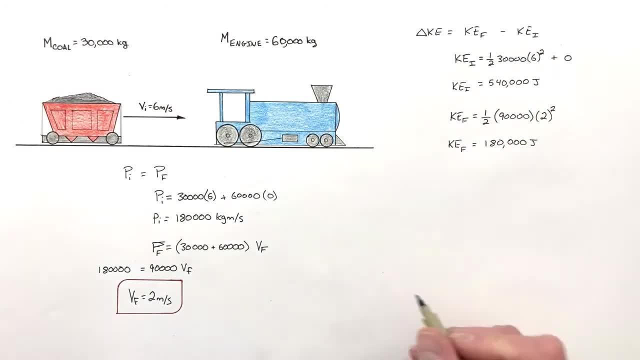 joules of kinetic energy And we'll put commas in there just to be good, little boys and girls. Now in solving for our overall change, It's gonna be 500.. Sorry, 180,000.. That's our final Minus 540,000.. 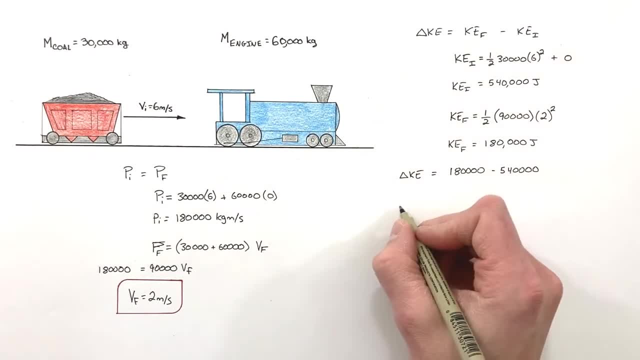 Minus 540,000.. Minus 540,000.. the initial kinetic energy and the overall change in kinetic energy is negative 360,000 joules. All right, let's talk about what this means, because there's some absolutely enormous.